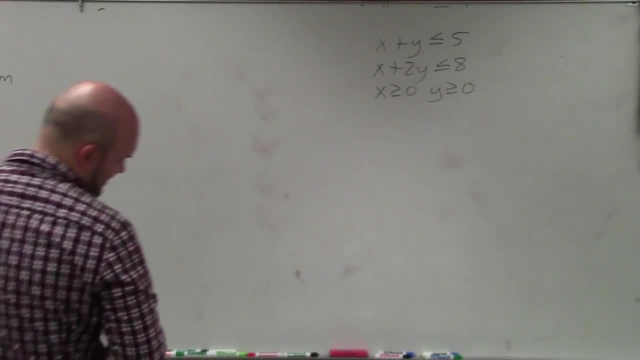 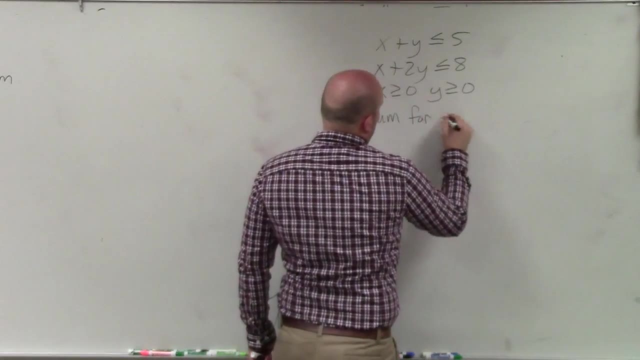 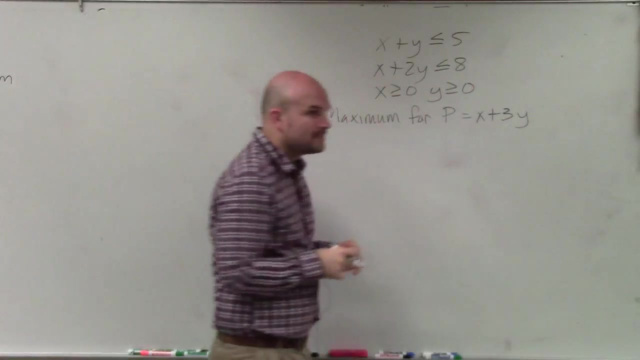 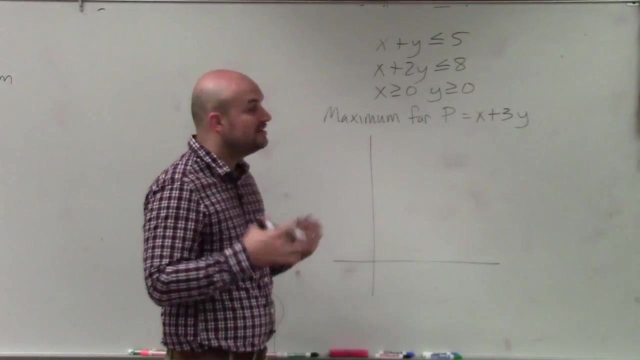 When you're given a problem like this and they want you to find the maximum for our objective equation is x plus 3y. So what I explained last class period and what I'd like you guys to do is, before you get into anything with linear programming, the main important. 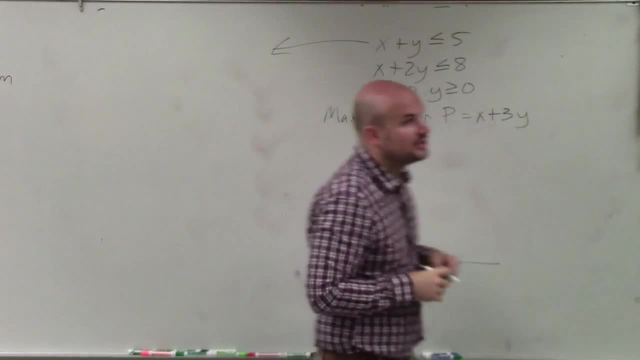 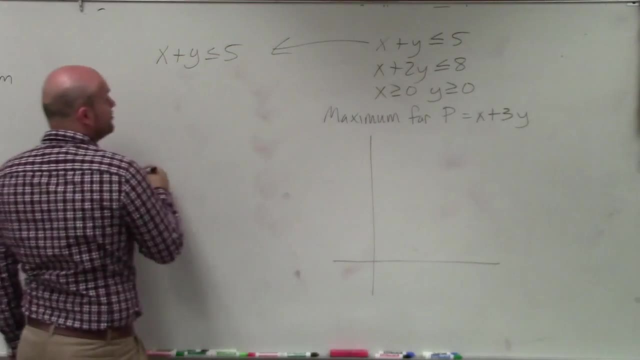 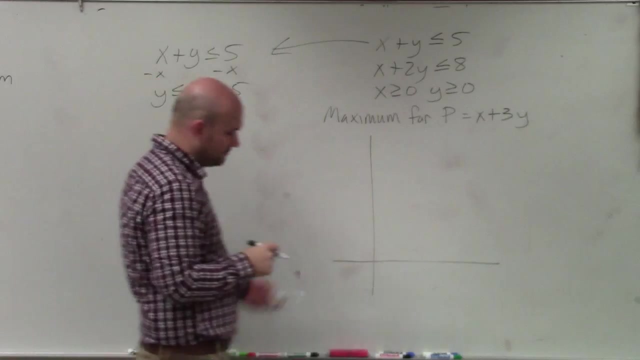 thing is just to graph each one of your linear inequalities. So, when graphing our linear inequalities, the best thing that I like to do is rewrite my linear inequality in slope intercept form. So I'm going to do that for each one. Now, the one mistake that I saw, a 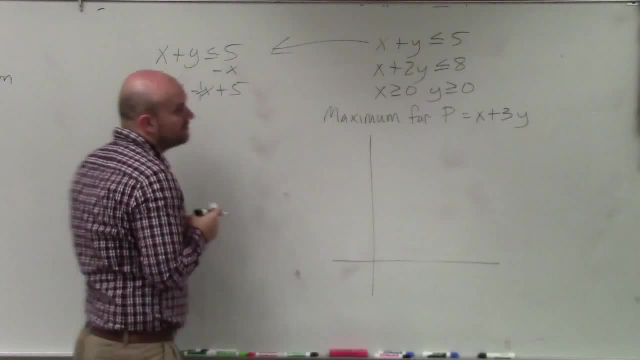 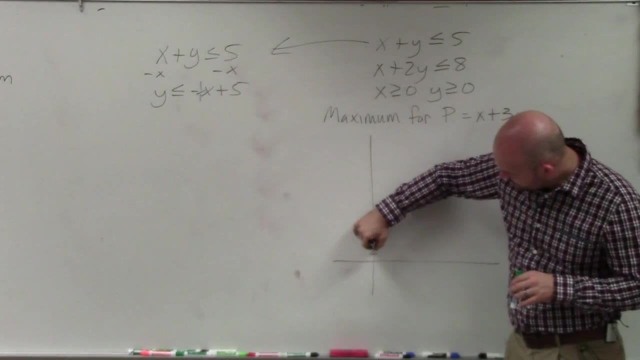 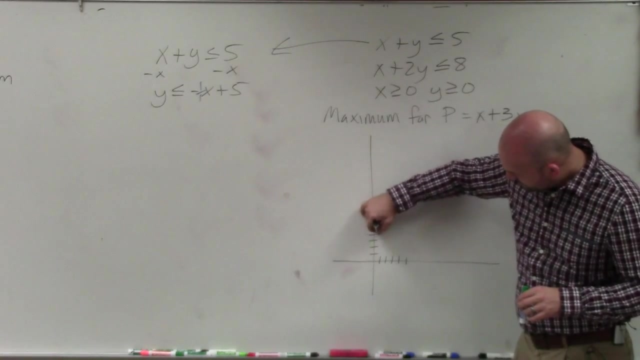 lot of students doing is they forgot that the slopes were negative, So they were going like down and to the left Over here. if I was going to graph this, I'm going to go up to 5.. 1,, 2,, 3,, 4, 5.. And I'm going to go down: 1, over 1.. 1,, 2,, 3, 4, 5.. Down: 1, over 1. Down. 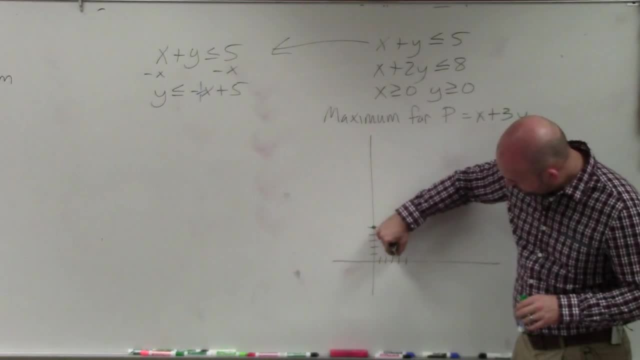 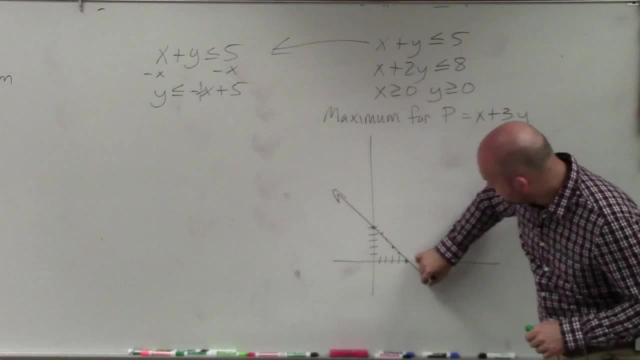 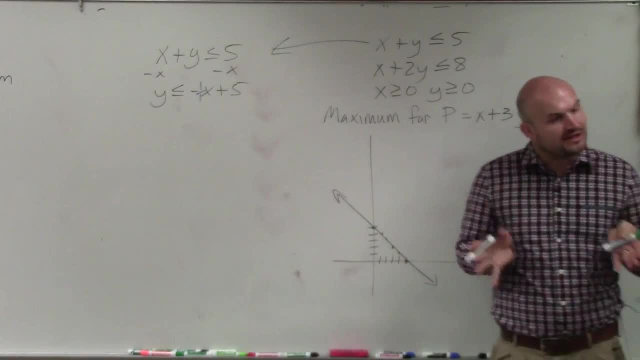 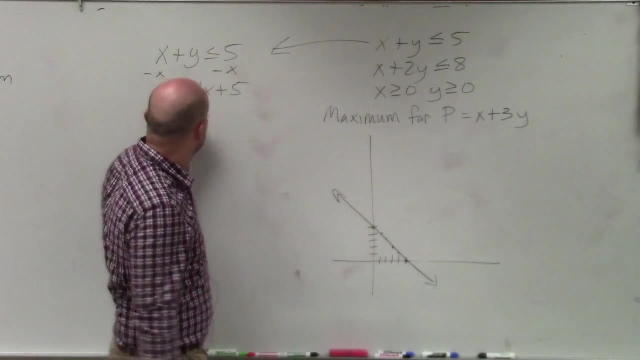 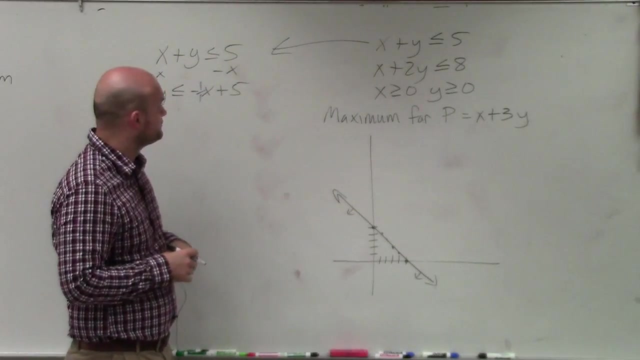 with grading, They're shading the whole thing. When you're graphing more than two inequalities, just use arrows and then shade the feasible. So it's less than right. So therefore, I'm just going to show myself two little arrows to say: hey, you're going to shade below that line. Then let's do the next one: x plus 2y. 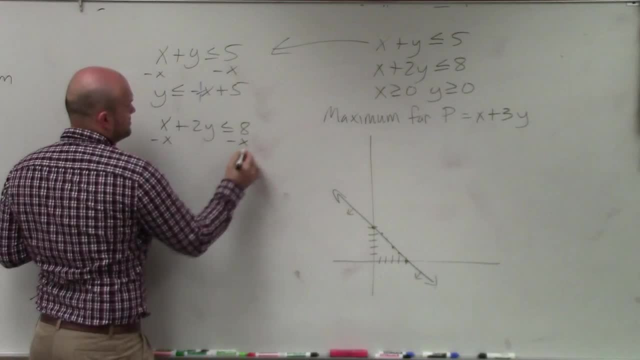 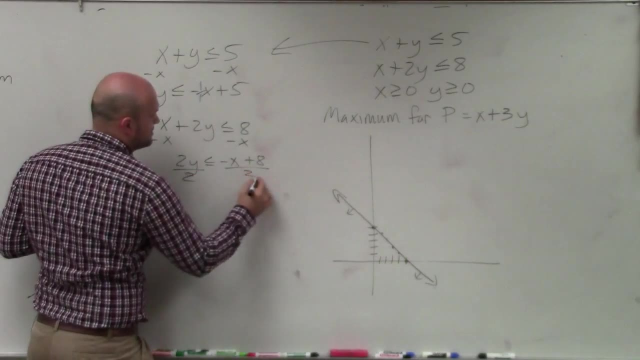 is less than or equal to 8.. Subtract x- Subtract x: 2y is less than or equal to negative x plus 8.. Divide by 2.. Divide by 2.. Remember the 2 goes into both of those And also remember: 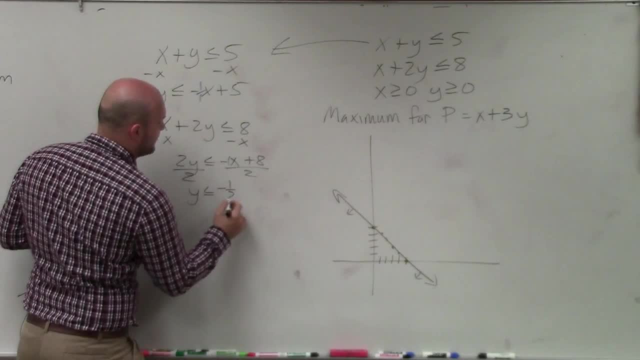 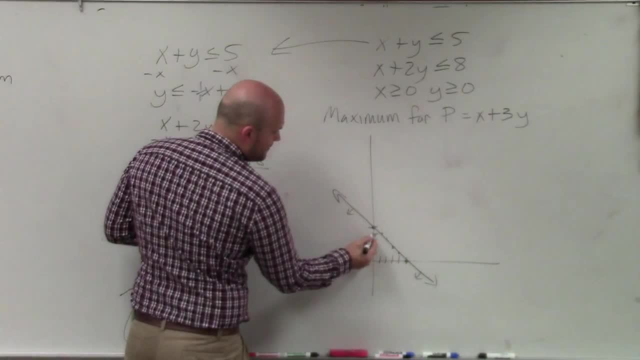 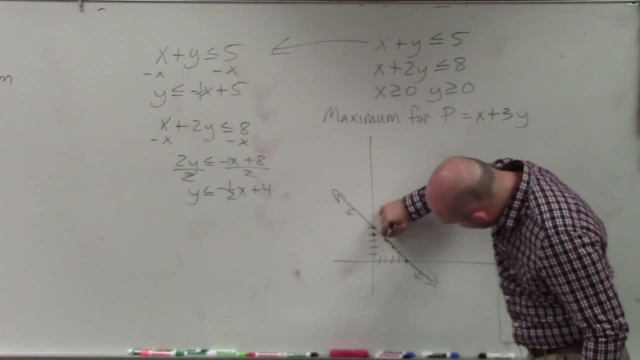 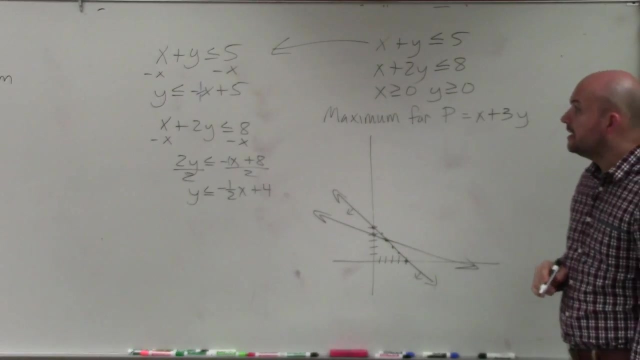 plus 4.. So now I'm only going to go up to 4.. And instead of going down 1, over 1,, I'm going to go down 1, over 2.. And then I'm just going to connect that line, OK, And then again, that's a less. 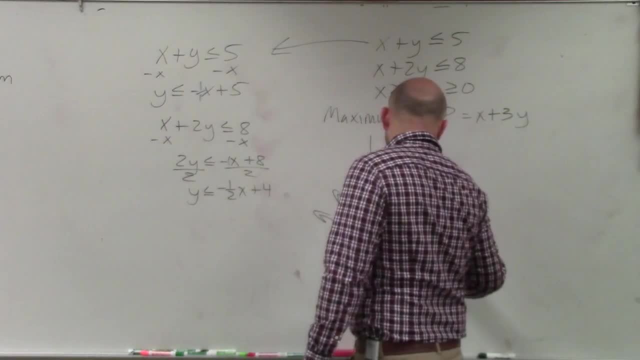 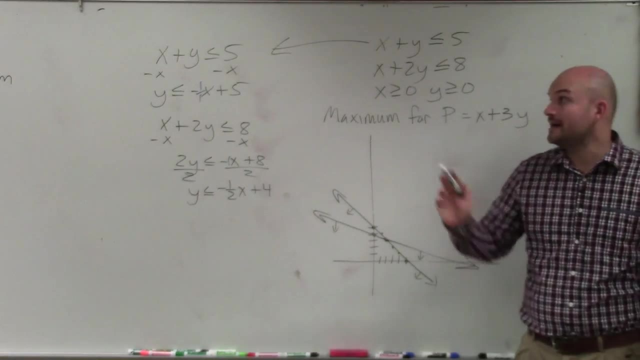 than or equal to. So I go down. I'm going to be shading down. Does anybody follow me or not? have any questions so far? So everybody good. So again, write your inequalities in slope-intercept form and graph and then shade. 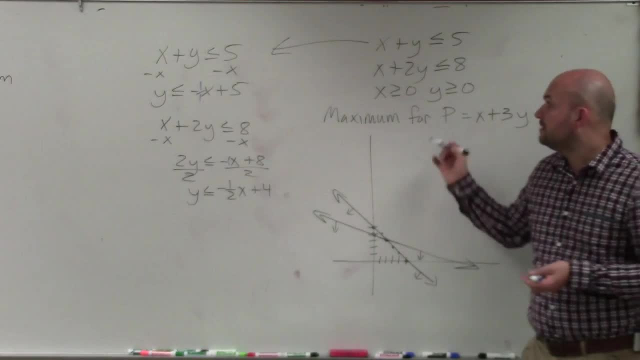 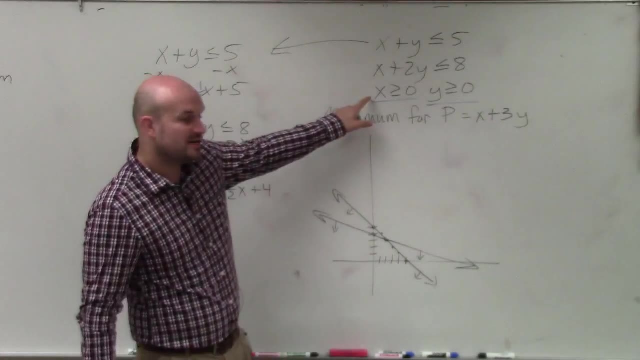 But just use the arrows. Right now we know everything's being shaded below. Then a lot of students had trouble with these: x is greater than or equal. y is greater than or equal to 0.. Well, x is greater than or equal to 0, guys. 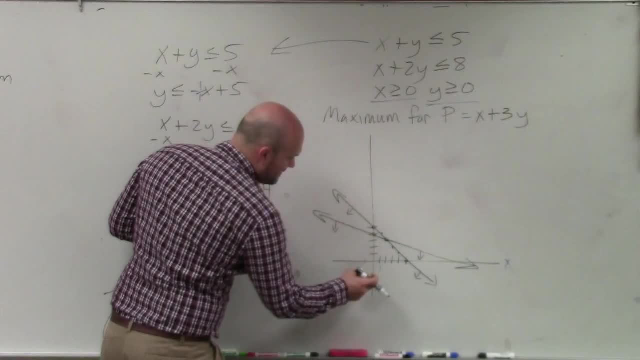 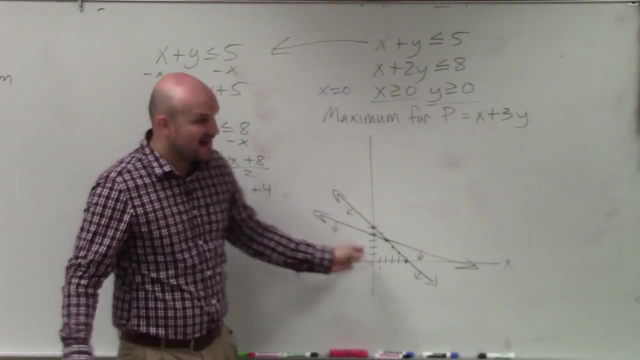 Remember, this is the x-axis. That's 1.. That's negative: 1.. That's 0.. When x, think of that as x equals 0.. That's when x equals 0.. That's going to be a vertical line. 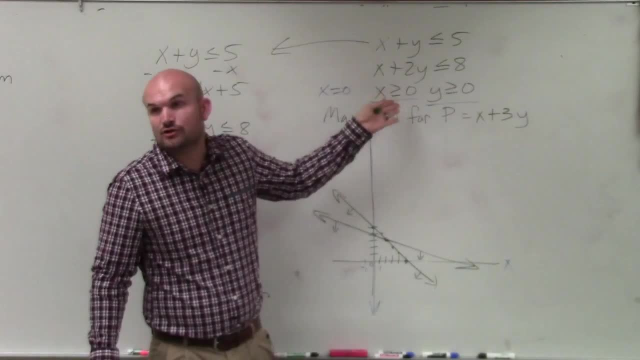 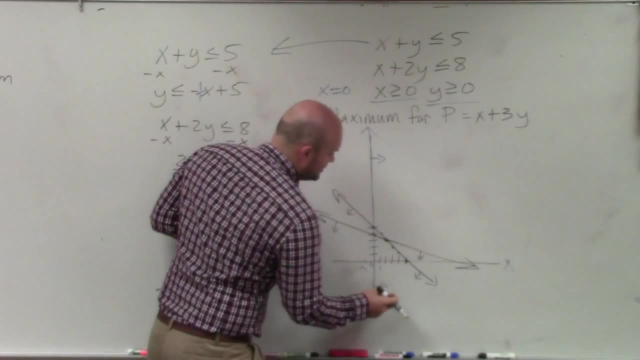 But it's saying they want you to shade for all values that are greater than or equal to 0. So that's going to be pointing to the right or to the left. To the right Again, I'm just going to use arrows. 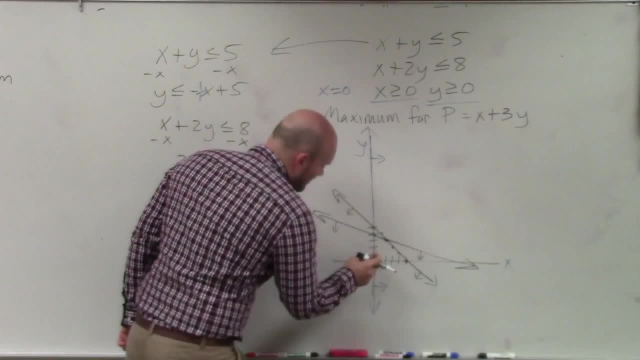 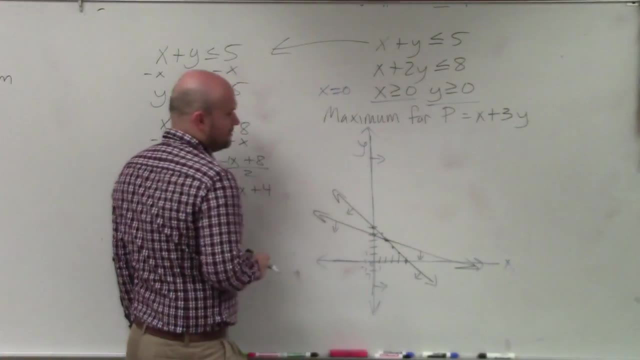 Then we have: y is greater than 0. This is the y-axis, That's 1.. That's negative 1.. That's 0. So that is a horizontal line. And then it's y. y is greater than so. that's going to be going up. 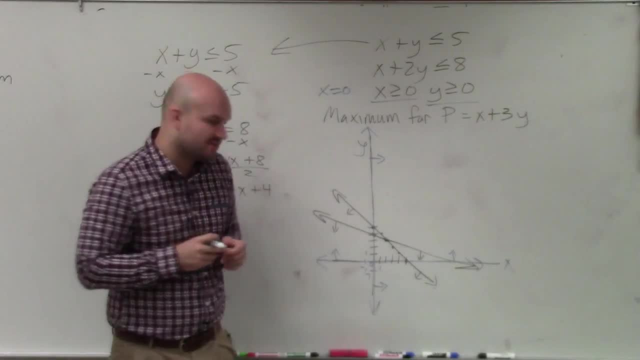 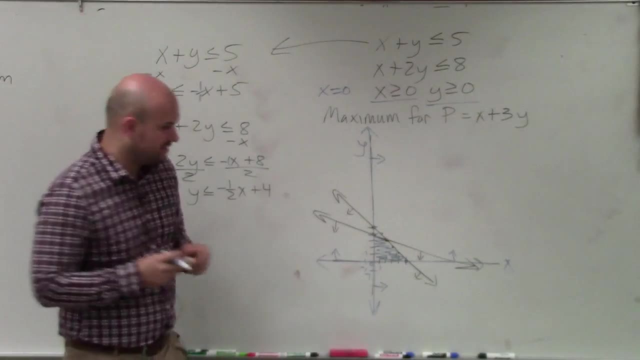 So hopefully you guys see, by looking at all of these arrows, you guys can see there's a feasible region which is right here And I'd like you guys to shade your feasible region. You don't need to label it, but you 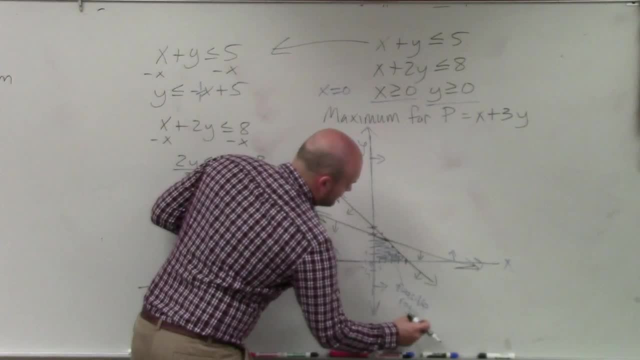 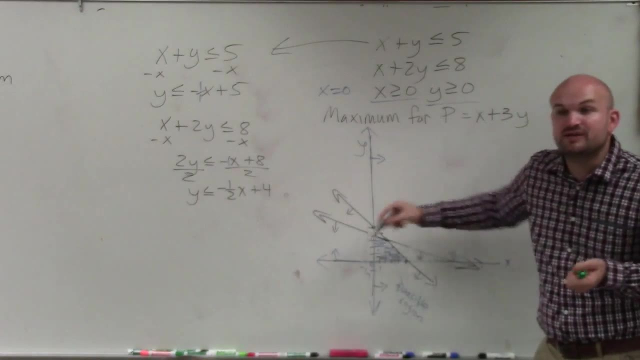 should know what that represents. Now of that feasible region. you can see that feasible region is bounded by 1,, 2,, 3, 4 boundary lines. You guys agree, those are lines. We call them boundary lines because they're. 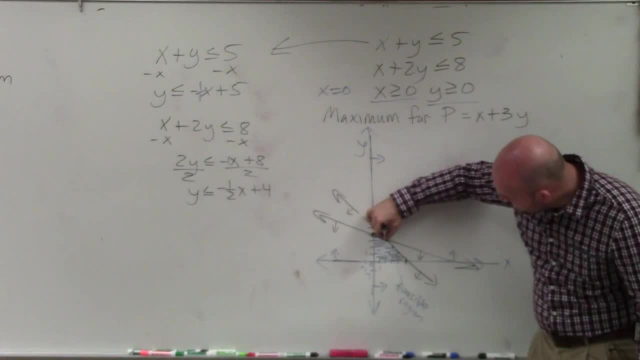 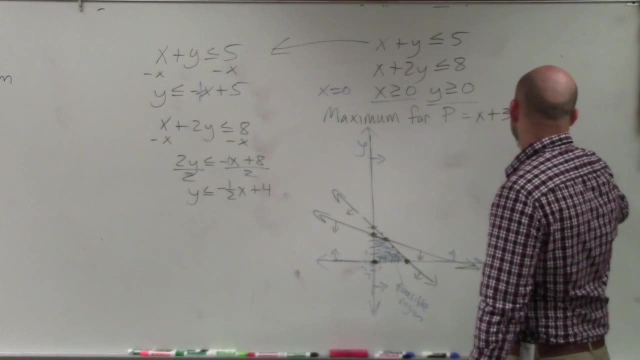 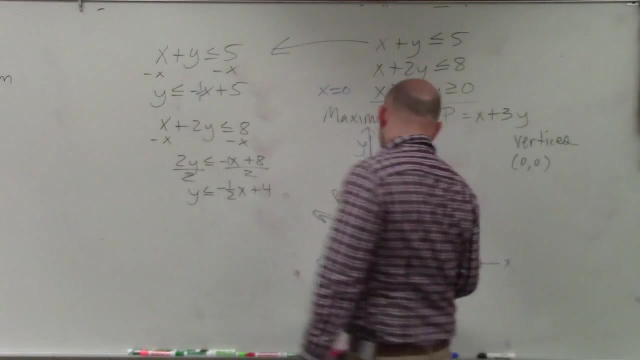 creating a boundary Well, where those boundary lines intersect on the feasible region, are what we call our vertices. So we'd say vertices. So our vertices are at 0 comma 0,, 0,, 1,, 2,, 3, 4.. 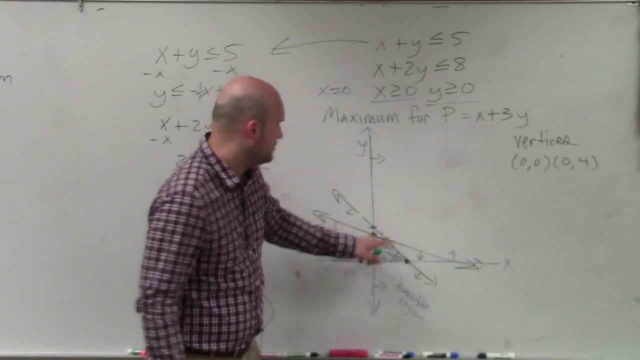 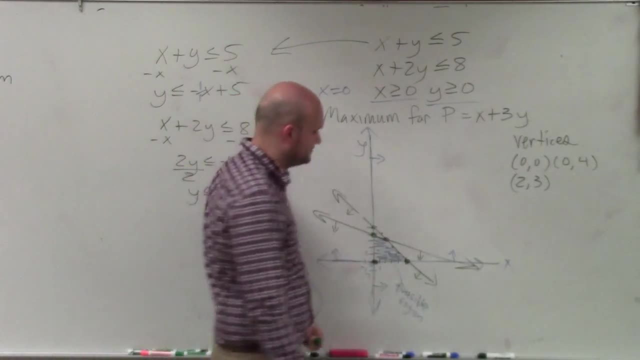 We have another at 2 comma, 1,, 2,, 3,, 4.. 3, and my last vertice is at 1,, 2,, 3,, 4,, 5,. OK, Even though this is another intersection. 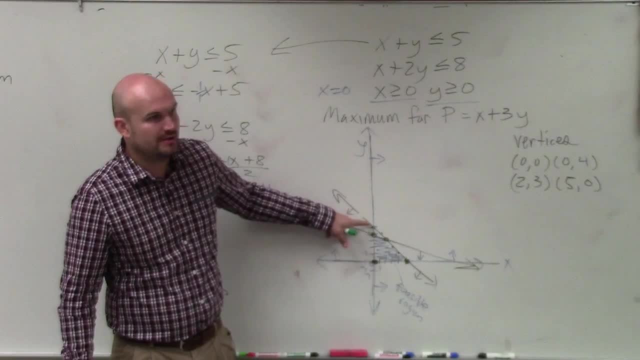 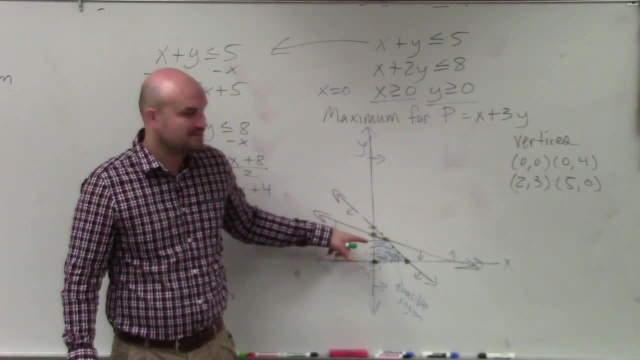 it's not on the feasible region, So we're not going to include that one. We only include the vertices that are on the feasible region. Does that make sense? Yes, A little bit. Less or minus. OK, Now we need to maximize the objective function. 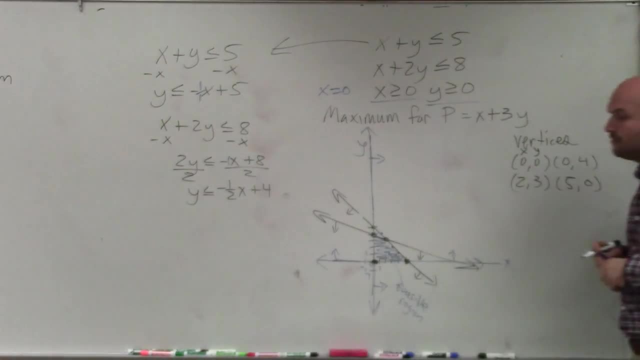 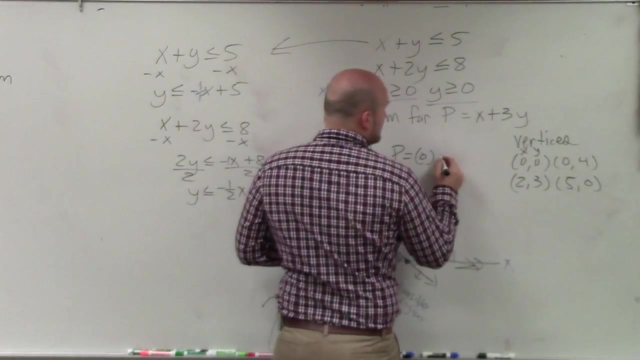 So you guys can see that each of these coordinate points is an x and a y coordinate point. Now all we're simply going to do is plug in x and y into my objective function and we're going to determine which one gives us the maximum value. 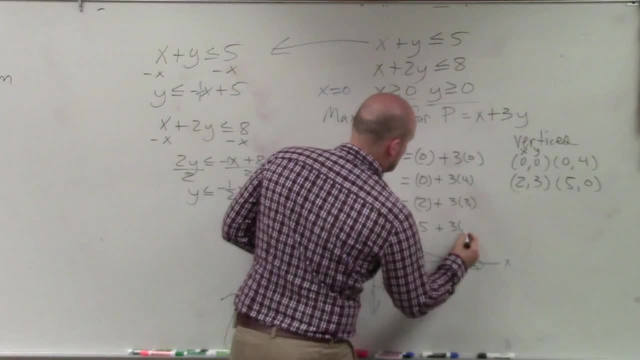 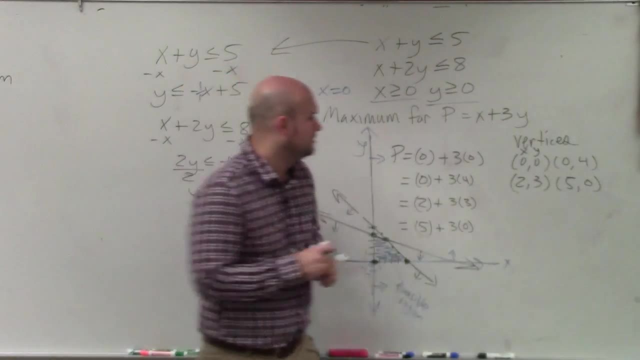 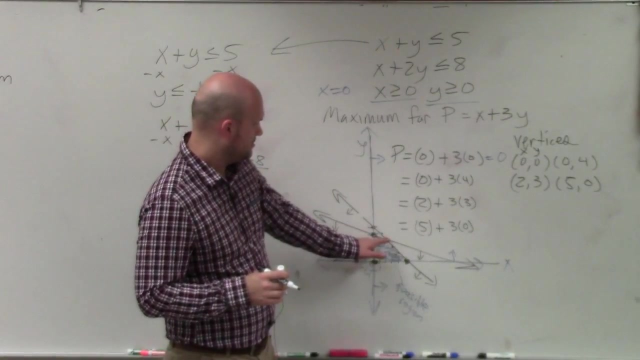 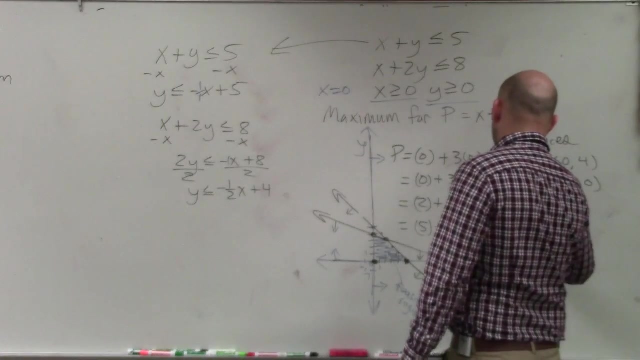 Does everybody see how I plugged in each value in for x and y of the objective function And we get it's what, Yes, that does produce my maximum. Oh wait, no, No, it doesn't. Yeah, it's 0, 4.. 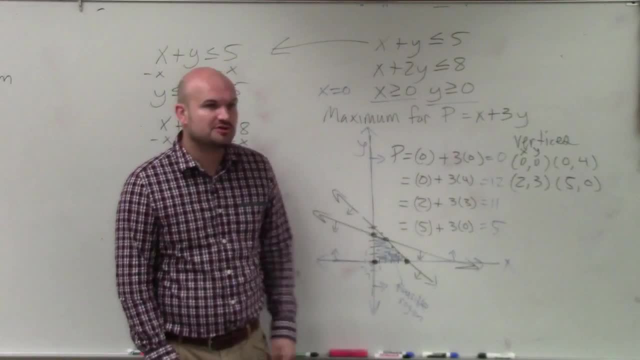 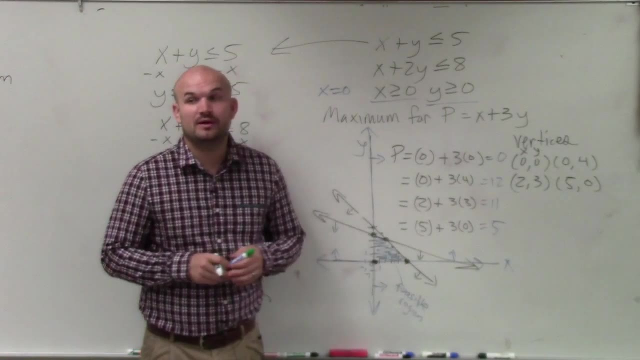 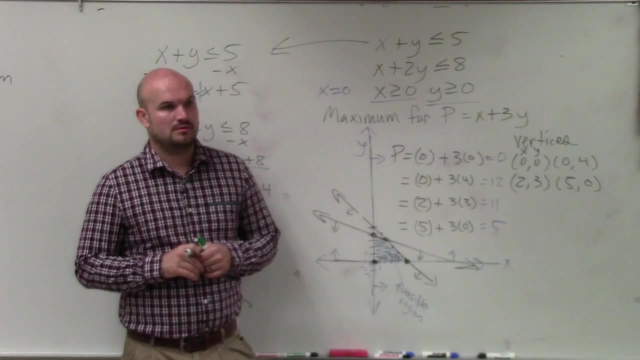 It's close, though It's very close, But that actually produces my maximum. Anybody have any questions on that? Make sure your 8 is correct, especially if you had missing work from there. Yes, So when I go back, I got the 8 times when I did it. 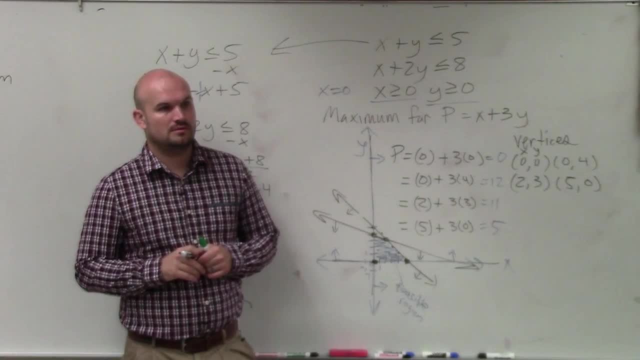 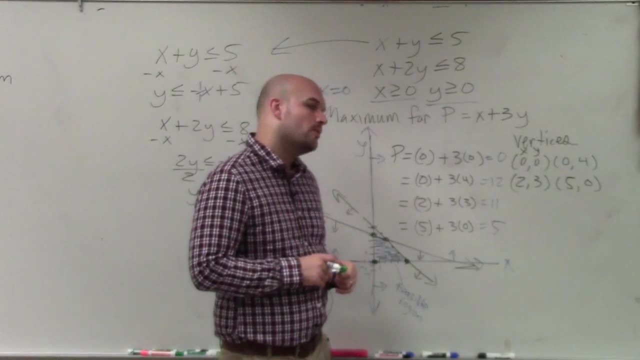 but it doesn't. I can't tell what my. So I got 3 of them right and then I got. I didn't get the 5, 0 thing, but I still got the maximum. So I would recommend I did some videos. 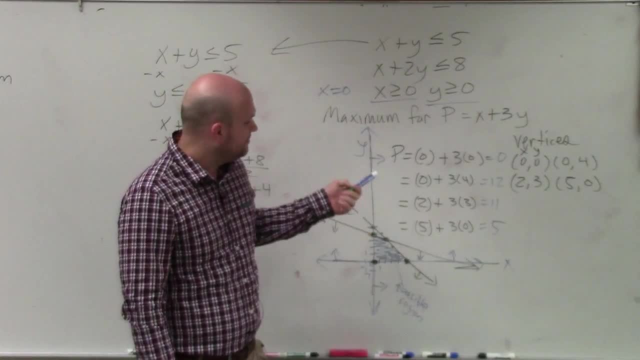 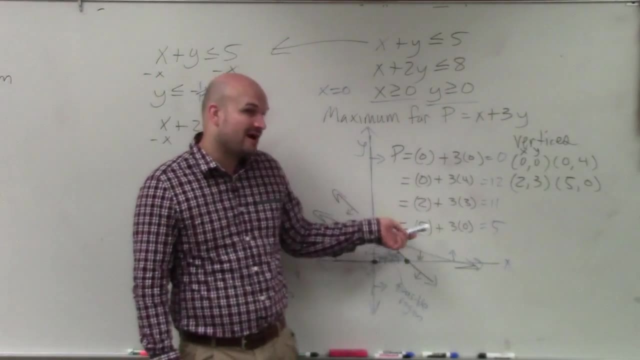 When you're graphing like- not on graph paper- you're not always going to have the exact vertices corrected. Also, even if you do have on graph paper, you might have vertices that are in between integers right, So you might have a fraction as an integer. 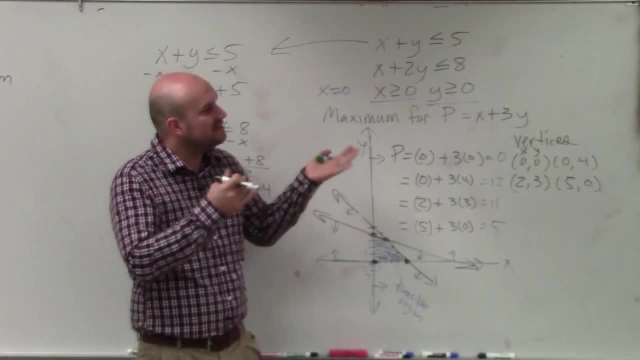 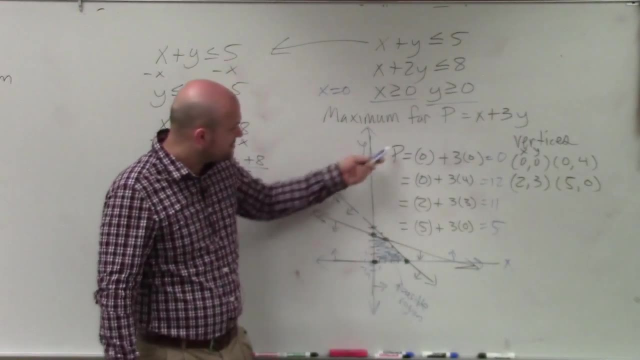 So you're just going to have to estimate to the best of your ability, Obviously like on a test or something you're not going to be. I would just say: be careful as you can Like, for instance, when the slope is down, 1 over 1,. 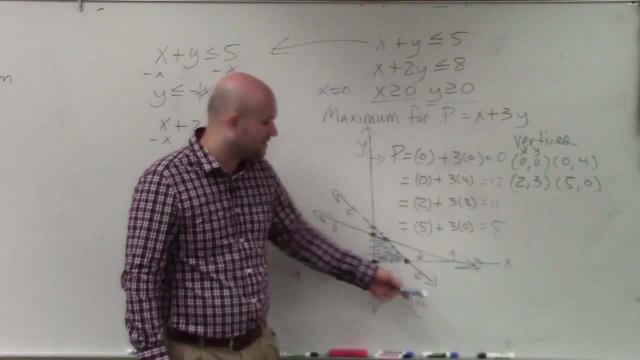 you can see I went down 1 over 1.. Down, 1 over 1.. I continue that pattern so I could see all these different points that lie on the line. OK, But it's OK if you're a little bit off.